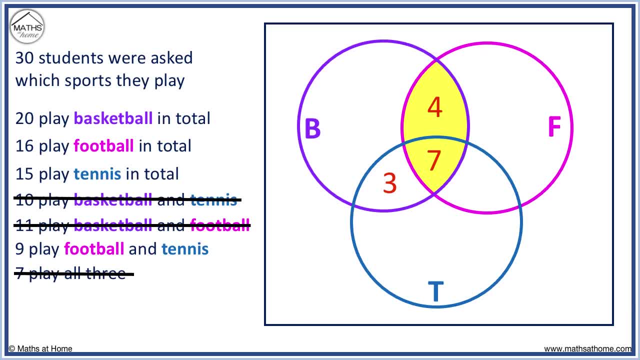 We need four more. here We cross off this information. Now nine people play football and tennis. That is this region. We have seven and need two more to make nine. Now we have looked at all overlap regions of two sports. Now we look at totals of each individual sport. 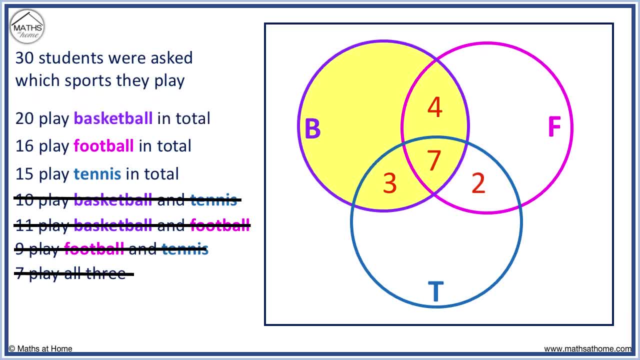 Twenty play basketball, which means the numbers in this circle need to add to twenty. We have three plus seven, which equals seven. Three plus seven equals ten, plus four equals fourteen. We need six more people to make twenty. Sixteen people play football. Four plus seven equals eleven, and eleven plus two equals thirteen. 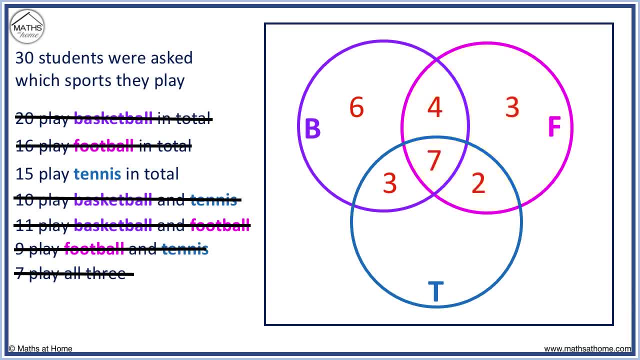 We need three more to make sixteen. in total, 15 play tennis. 3 plus 7 plus 2 equals 12.. We need 3 more to make 15.. Finally, we know that 30 students were asked in total. All of our numbers must add to 30 in total. 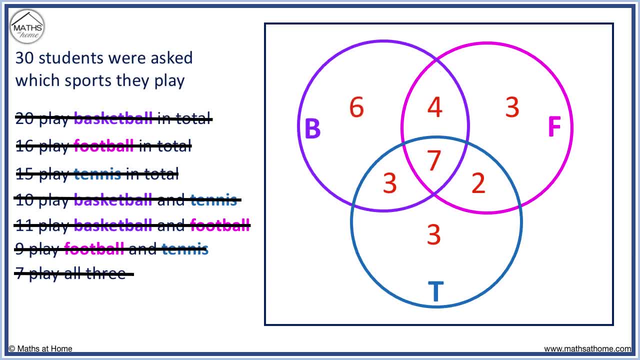 6 plus 4 equals 10,, plus 3 equals 13,, plus 7 equals 20,, plus 3 equals 23,, plus 2 equals 25, and plus 3 equals 28.. We don't have 30. We need 2 more. 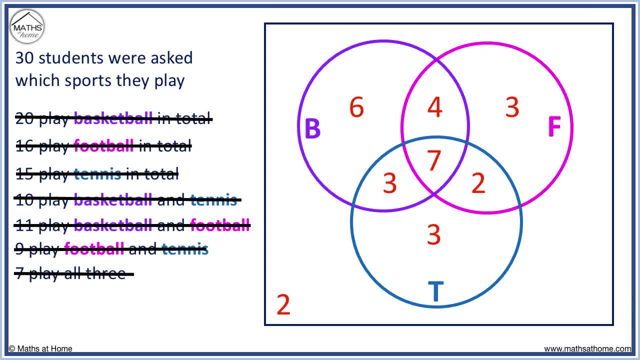 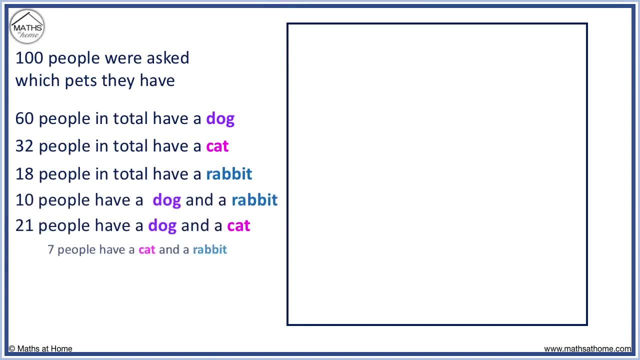 These 2 students go on the outside of all the circles because they do not play the 3 sports of basketball, football or tennis. Here is a new question which we will draw a Venn diagram for. We have a circle for each pet listed: Dogs, cats and rabbits. 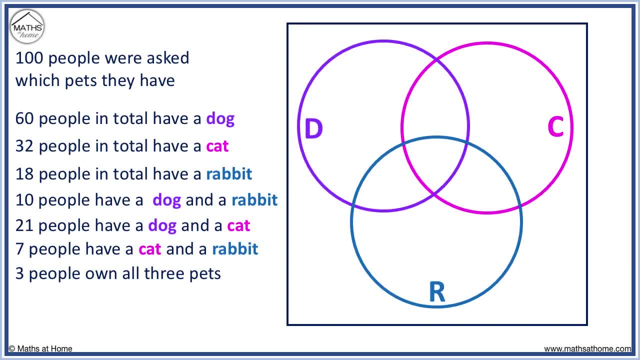 We start with the overlap of all 3 circles. 3 people own all 3 pets. This goes in the overlap of the 3 circles. Now we look at the overlap of 2 pets: 10 have both a dog and a rabbit. 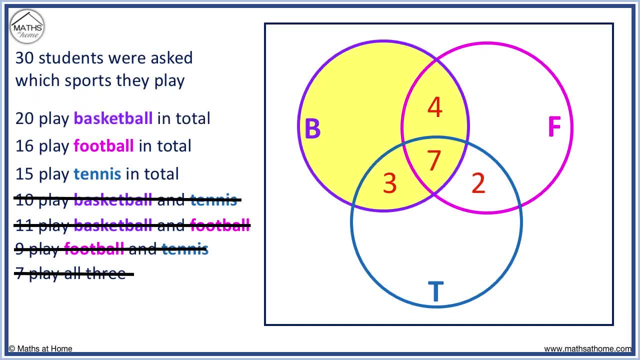 Twenty play basketball, which means the numbers in this circle need to add to twenty. We have three plus seven, which equals nine. We have three plus seven, which equals ten, plus four equals fourteen. We need six more people to make twenty. Sixteen people play football. Four plus seven equals eleven, and eleven plus two equals thirteen. 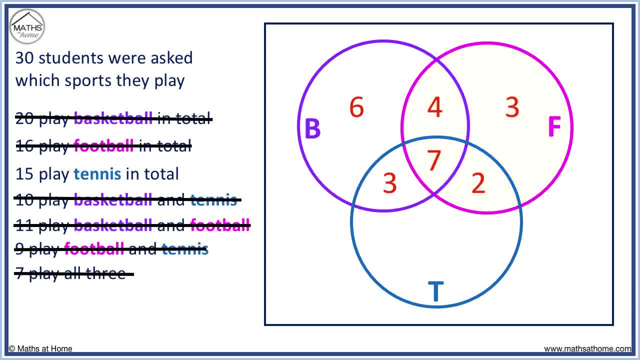 We need three more to make sixteen. in total, Fifteen play tennis. Three plus seven equals ten. Three plus seven plus two equals twelve. We need three more to make fifteen. Finally, we know that thirty students were asked in total. All of our numbers must add to thirty in total. 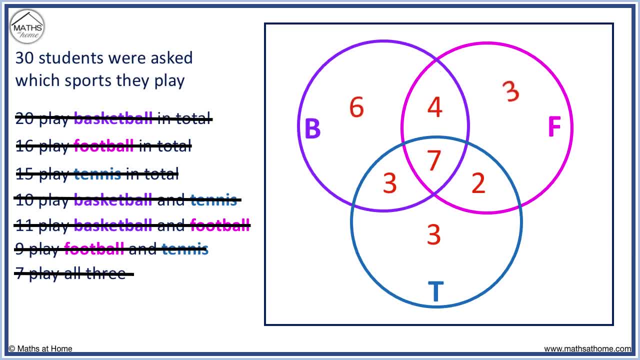 Six plus four equals ten, plus three equals thirteen. plus seven equals twenty, plus three equals twenty-three. plus two equals twenty. Two plus three equals twenty-five, and plus three equals twenty-eight. We don't have thirty, We need two more. 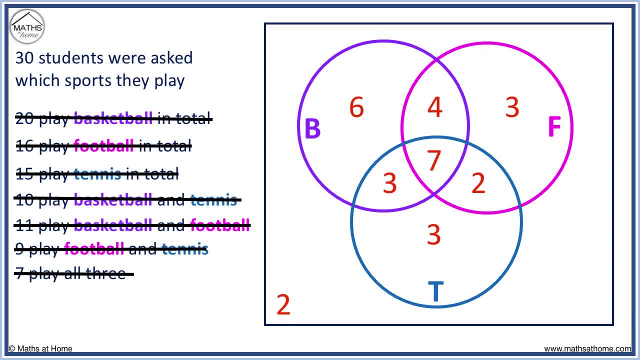 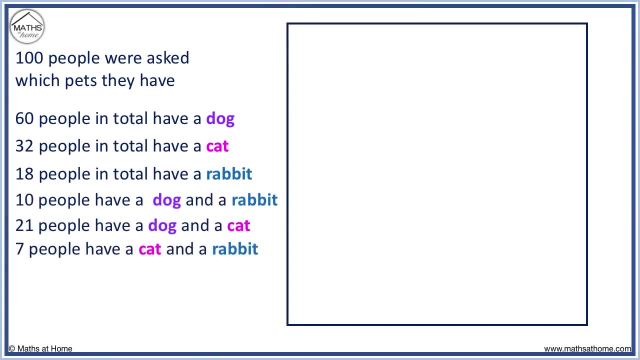 These two students go on the outside of all the circles because they do not play the three sports of basketball, football or tennis. Here is a new question which we will draw a Venn diagram for. We have a circle for each pet listed: Dogs, cats and rabbits. 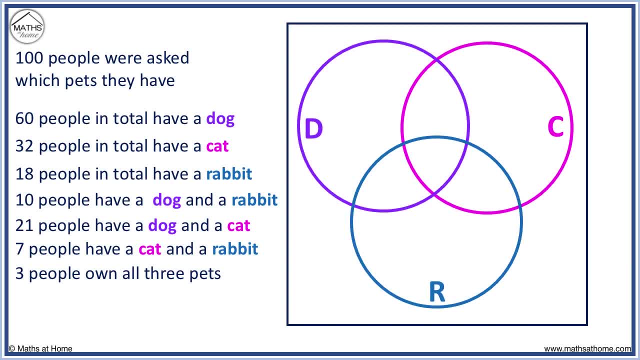 We start with the overlap of all three circles. Three people own all three pets. This goes in the overlap of the three circles. Now we look at the overlap of two pets. Ten have both a dog and a rabbit. Here is the overlap. 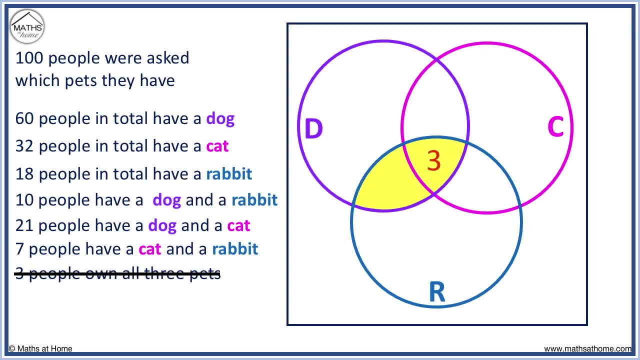 And we have three already. We need seven more. Twenty-one people have a dog and a cat. We have three and need eighteen more to make twenty-one. Seven people have a cat and a rabbit. We have three and need four more. Now we look at the totals in each individual circle. 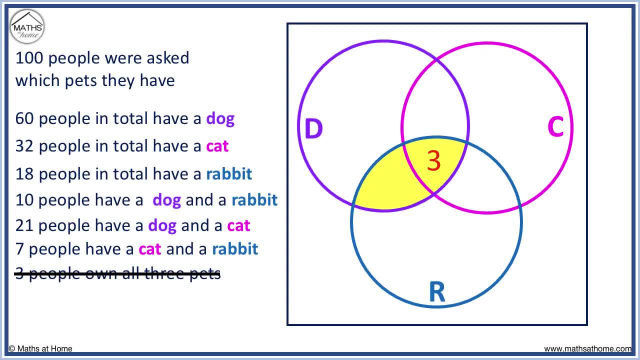 Here is the overlap: and we have 3 already. We need 7 more. 21 people have a dog and a cat. We have 3 and need 18 more to make 21.. 7 people have a cat and a rabbit. 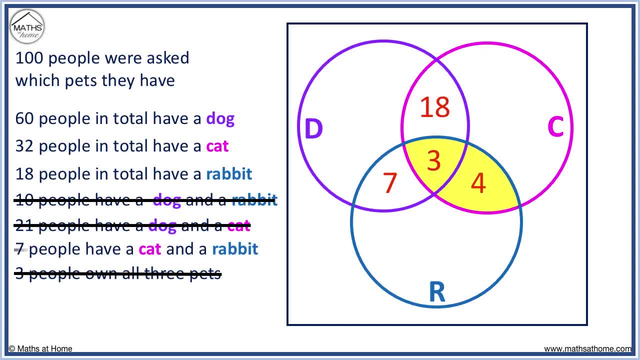 We have 3 and need 4 more. Now we look at the totals in each individual circle, 60 people own a dog. We have 7. plus 3 equals 10, plus 18 equals 28.. We need another 32 to make a total of 60 in the circle. 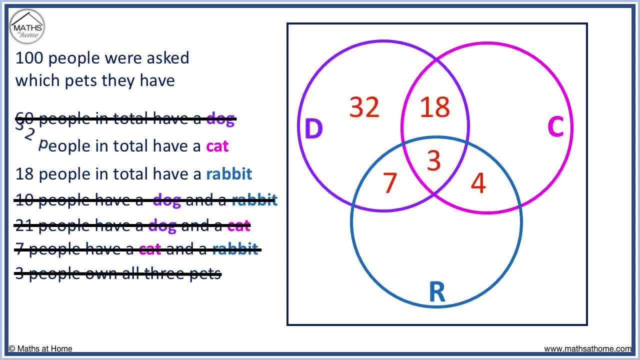 32 people have a cat. Already we have 4 plus 18, which equals 22,, and plus 3 equals 25.. We need 7 more to make a total of 32.. Now, 18 people have a rabbit. 7 plus 3 equals 10, plus 4 equals 14.. 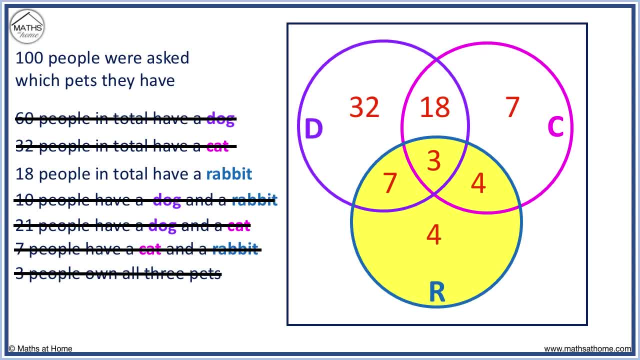 We need 4 more to make 18.. Finally, we know that the numbers must add up. The numbers must add to 100.. 32 plus 18 equals 50, plus 7 equals 57, plus 3 equals 60, plus 7 equals 67, plus 4 equals 71, plus 4 equals 75.. 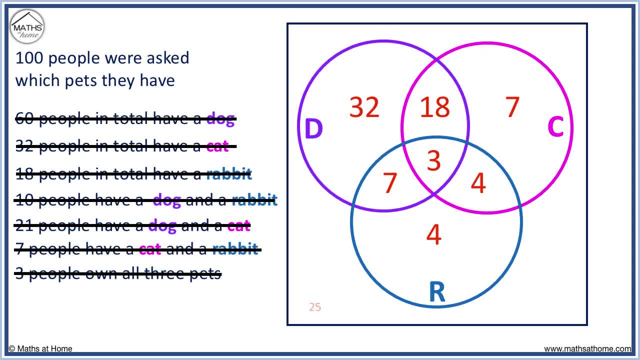 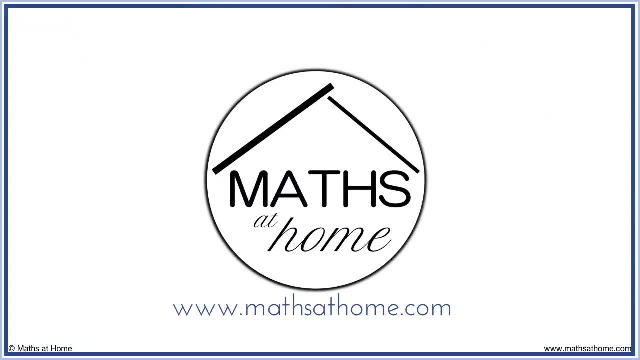 We have 75 people so far, so we need 25 more to make 100.. These people do not own any of the 3 pets, and so they are on the outside of the circles. Visit mathsathomecom for further videos and practice.